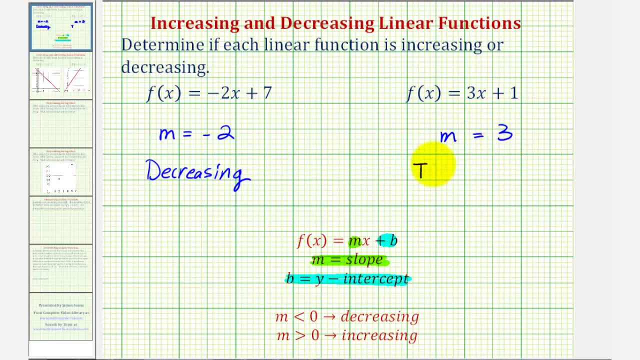 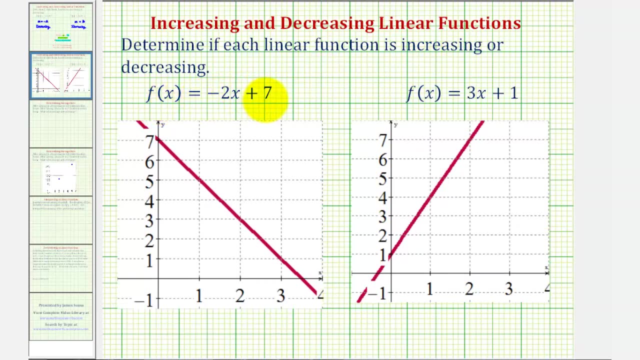 and therefore the linear function is increasing. Let's take a look at the graph of these two functions to get a better understanding of what it means for linear function to be increasing or decreasing. If we first consider, f of x equals negative two x plus seven. if we wanted to graph this, 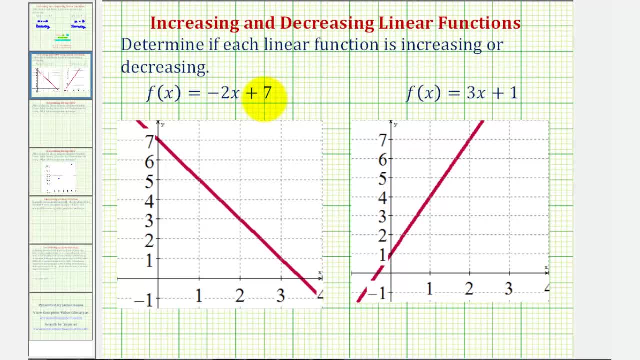 notice how the y-intercept is positive seven, which would give us this point here, and then again the slope is negative two, or if we want negative two over one. so from the y-intercept if we went down two units and right one unit, 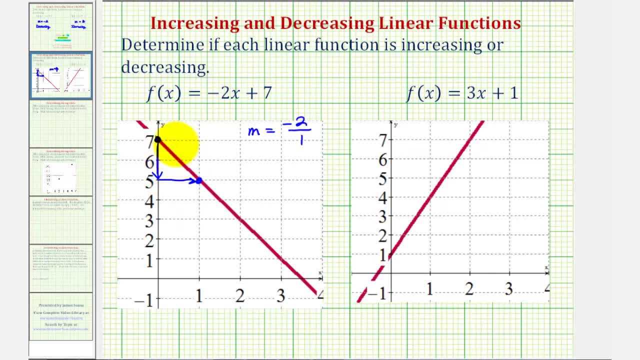 we have another point on the linear function. So notice how, as we move from left to right, the graph goes downhill and therefore the linear function is decreasing. We can also say that as x increases, y decreases. or, using our slope, notice that y decreases by two. 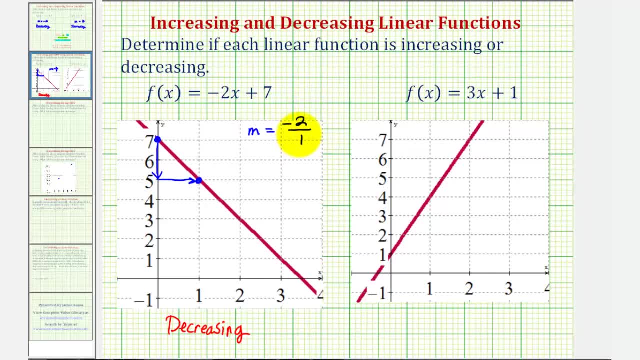 every time x increases by one. We know this because we have a negative two in the numerator and a positive one in the denominator. And remember, the slope of a line is the ratio of the change of y to the change of x, Or we could also say the change in the function value. 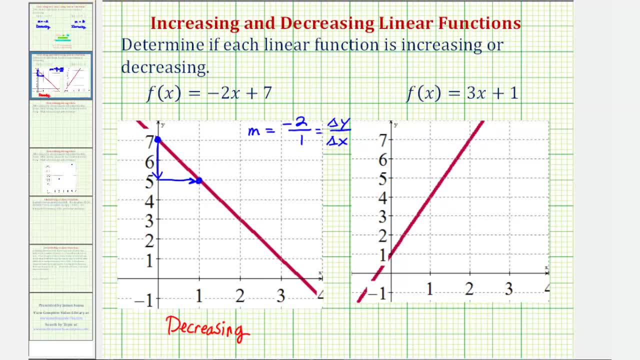 to the change in x. And then looking at the second linear function, f of x equals three x plus one. notice how the y-intercept is positive one, giving us this point here, And then, because the slope is positive, three, if we want three over one. 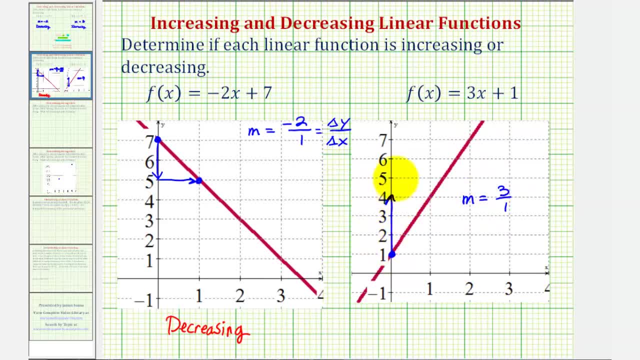 from the y-intercept. if we go up three units and right one unit, we have another point on the linear function And notice how the line is going uphill from left to right and therefore the function is increasing. We can also say as x increases. 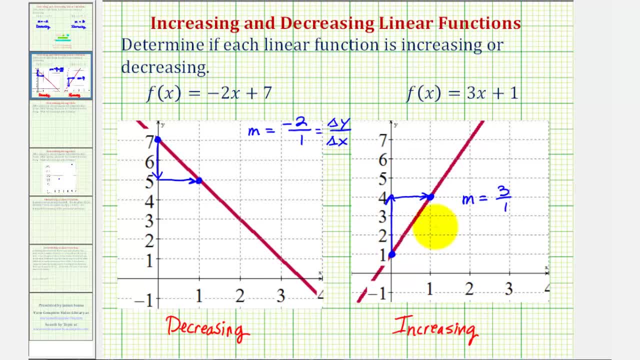 notice that y also increases. Or more specifically again, because the slope is the ratio of the change of y to the change of x. we can say the y value or function value increases by three every time the x value increases by one. I hope you found this explanation helpful.